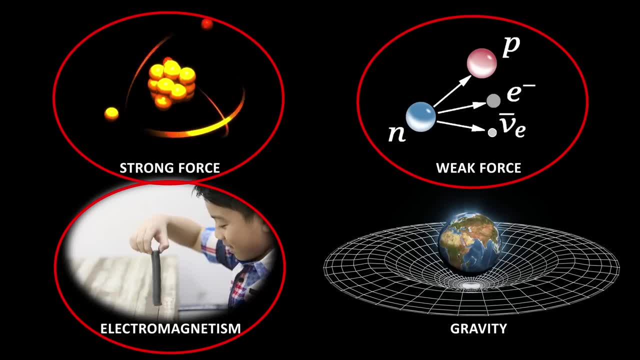 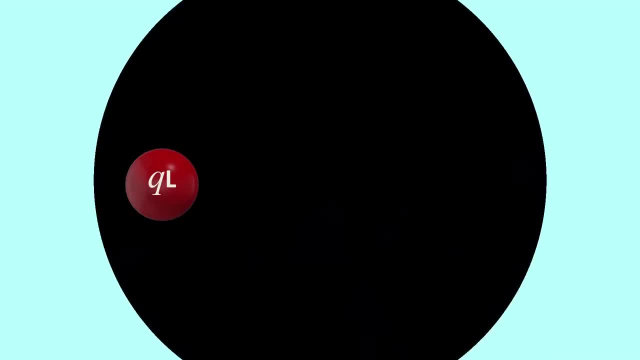 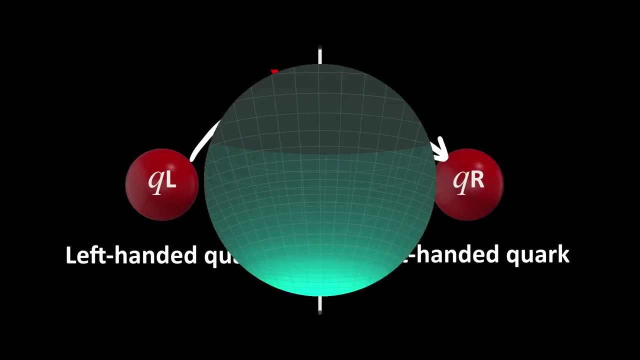 They lead to the electromagnetic weak and strong forces, as I showed in a prior video. However, as important as symmetries are, there is something that is at least as equally profound, And that is the fact that certain symmetries can be broken And without these broken symmetries, 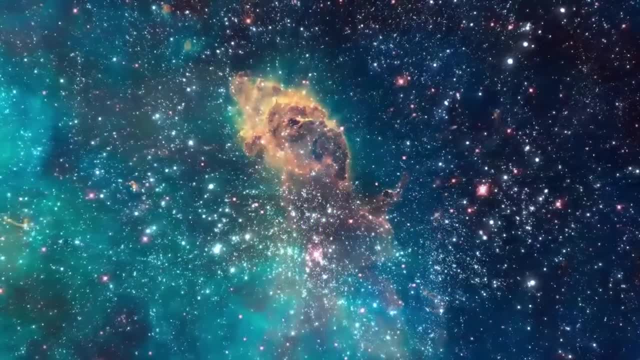 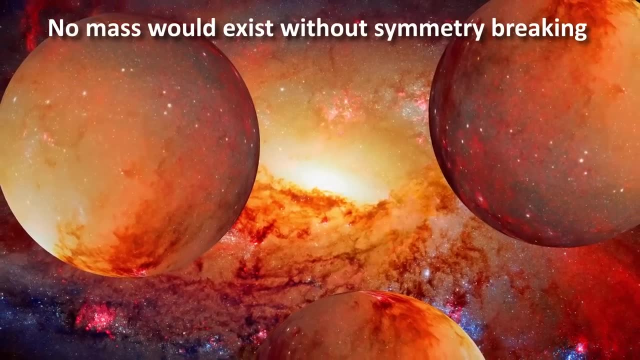 we would not have the universe that you and I are familiar with, And there would be no life as we know it. I am going to show you how no mass would exist in the universe without breaking symmetries. How can symmetries be fundamental if they can be broken? What are broken symmetries anyway? 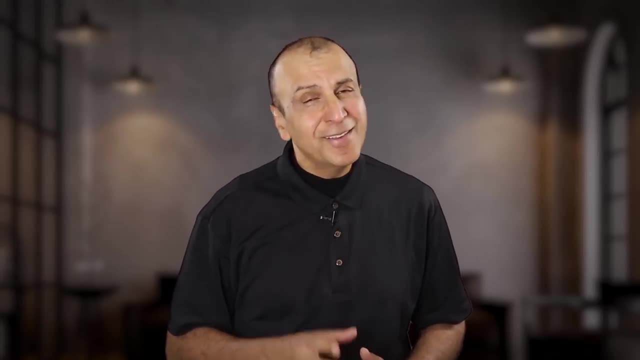 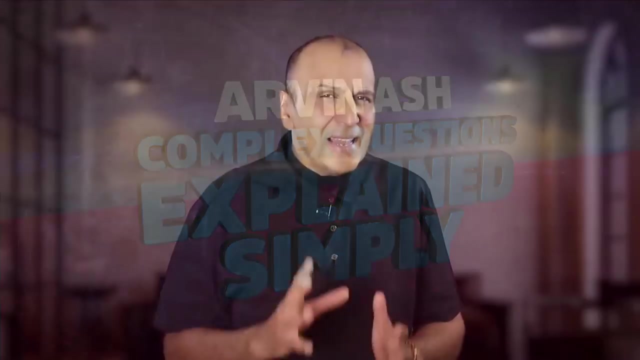 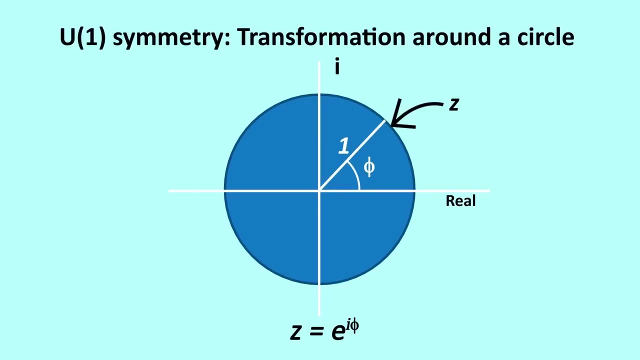 And what would the universe be like if we didn't have broken symmetries? That's coming up right now. Let's take a look at what symmetry is. A simple example is a mirror image. Symmetry in physics is when properties of particles don't change after being subjected to transformation or operations. 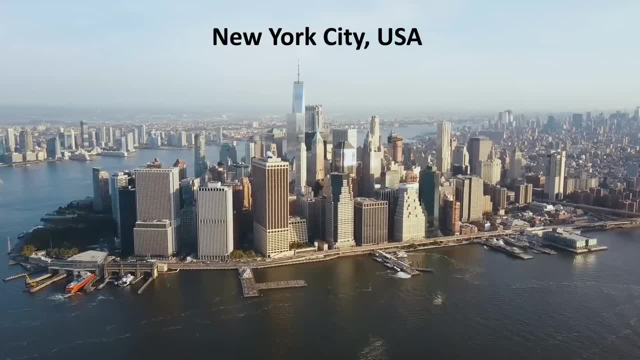 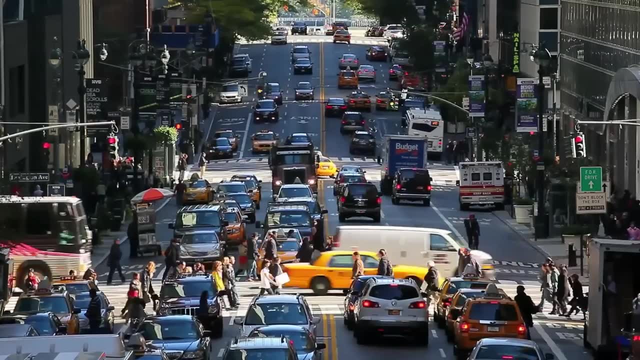 example, is the fact that the laws of physics are the same whether you are here or in China. This is space translation symmetry. Or the laws of physics are the same today as they were a hundred years ago. This is time translation symmetry. Symmetries like this show us that mother nature 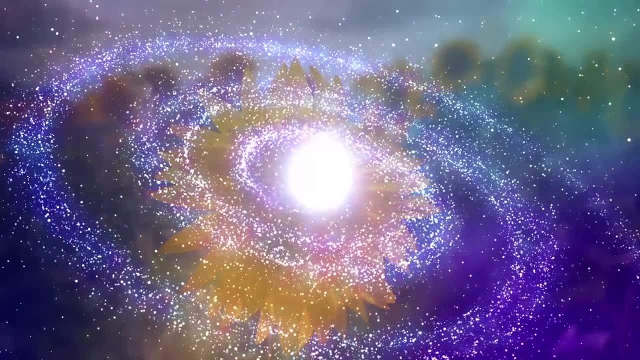 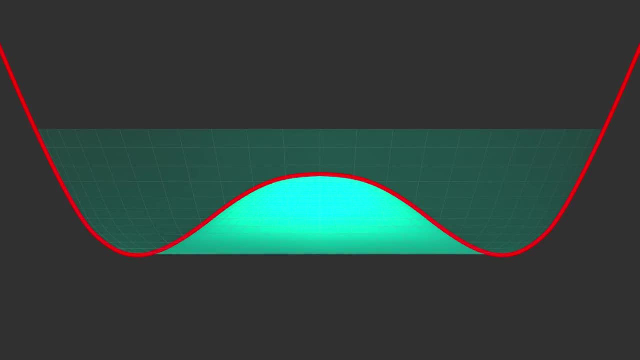 has some simple rules it uses to build the universe, but it also sometimes breaks certain of these rules. Consider the following graph, which depicts an energy potential. in physics, We have two minima, as shown on the left and the right side, and the maximum in the middle. 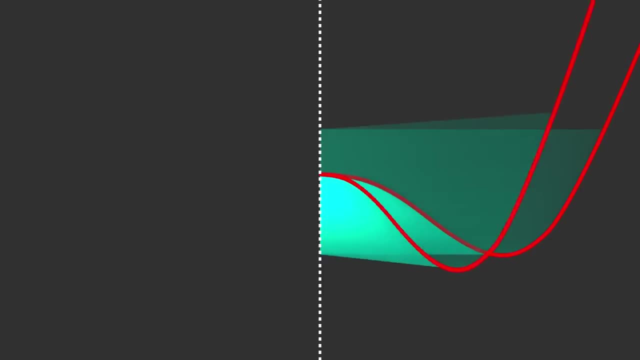 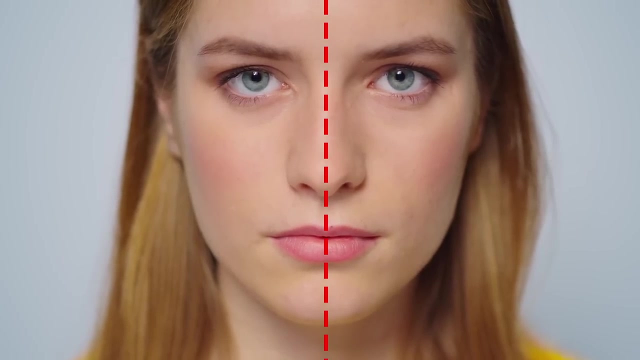 If we put a mirror vertically along the center, the mirror images are identical. In other words, the right side is equal to the left side. Again, this is similar to how humans are also symmetrical along the central vertical axis, at least externally, ignoring minor asymmetries. 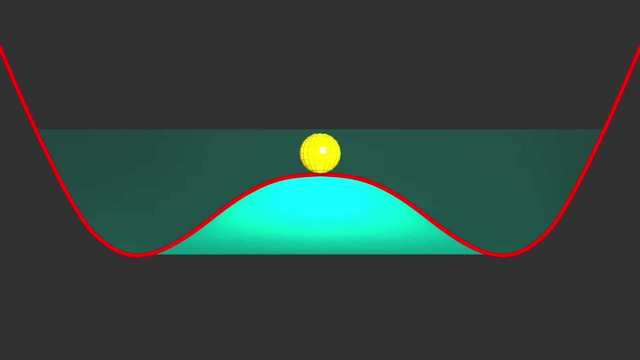 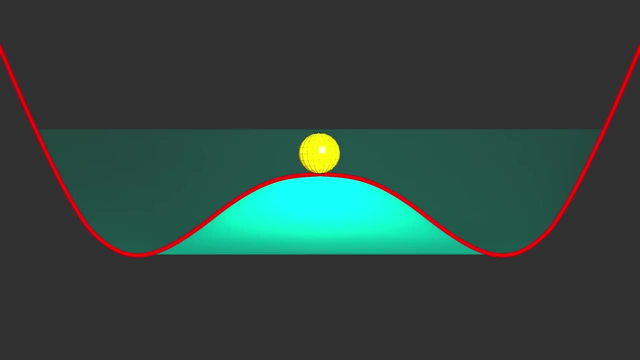 You would put it in the middle at the maximum, Because this way the mirror image would each contain half of the ball, such that combining the halves of the graph would lead to a complete round ball and the full graph. What if, instead, we put the ball in one of the minima, Let's say on? 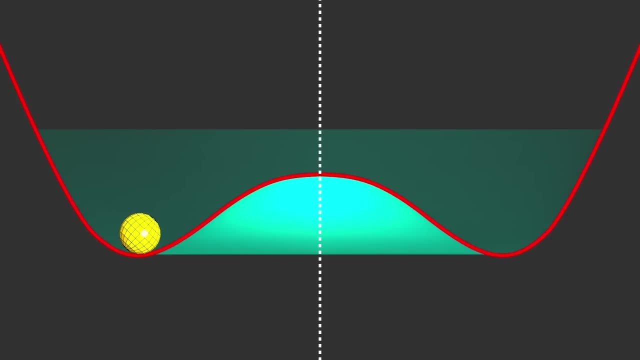 the left side. We again place a mirror in the middle. Now the mirror image of the left side doesn't represent what the graph really looks like. The symmetry no longer exists. The symmetry is broken if we put the ball there. Likewise, it would also be broken if we put the ball on the right side. 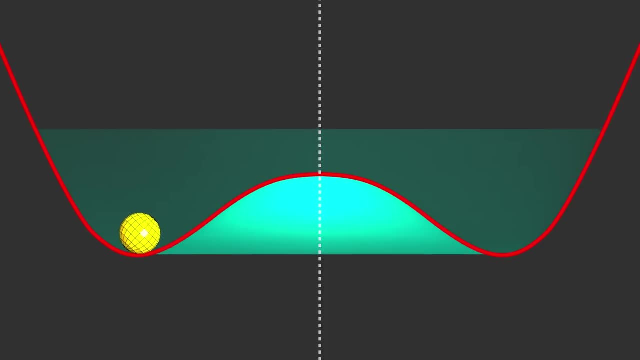 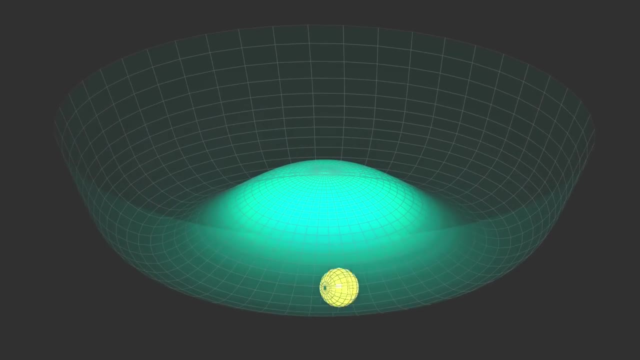 This is not just a random example. This is a visual representation of how the Higgs mechanism works to impart mass to fundamental particles. Certain fundamental particles break symmetry by not being in the center, by being in the non-zero potential of the Higgs field. I made a video on this. 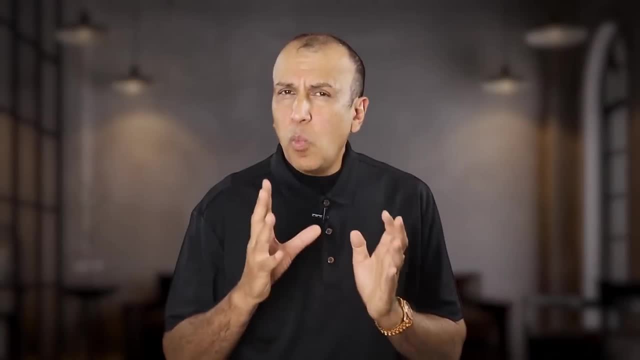 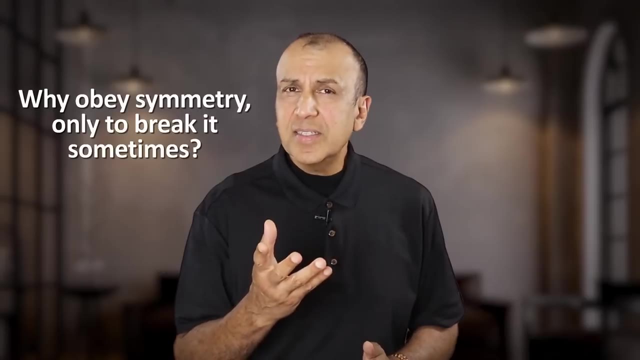 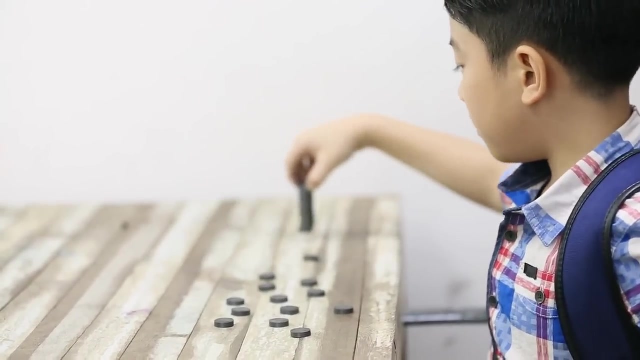 here if you want to find out more. But why does the universe appear to obey certain fundamental symmetries, only to sometimes break them? Why is it inconsistent? Well, we don't have a satisfactory answer for this question, other than to say that the universe wouldn't work the way we observe it. 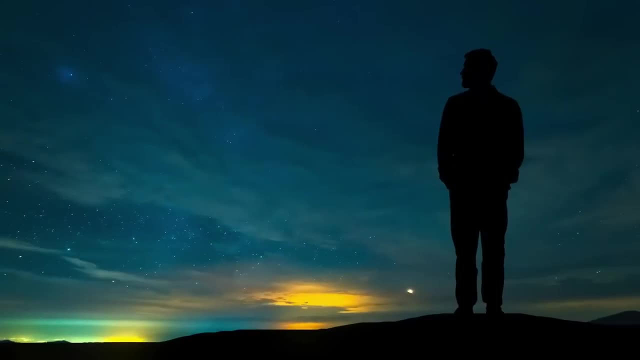 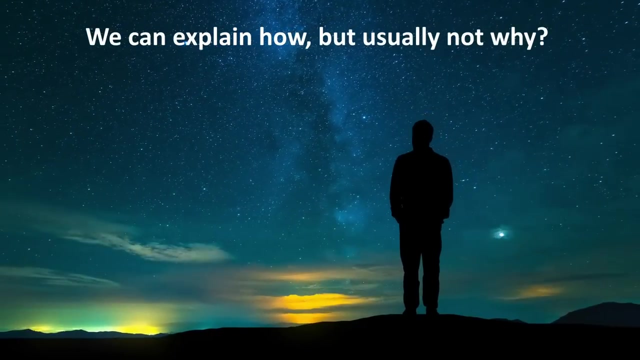 to work without symmetry breaking And, unfortunately, why questions are rarely, if ever, answered. in physics, We can explain how things work very well, but not why Symmetry breaking must occur in order to explain any mass in the universe, which is clearly what. 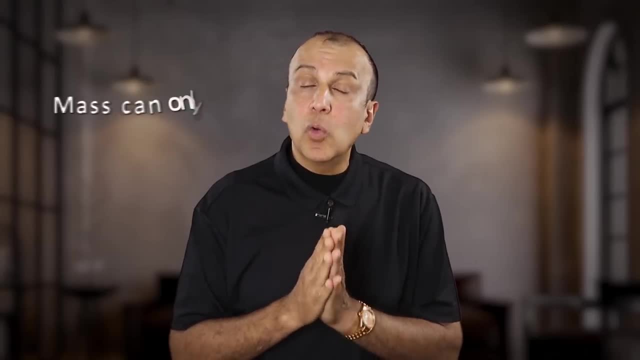 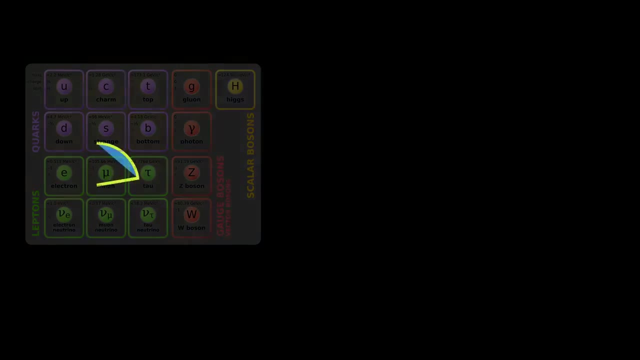 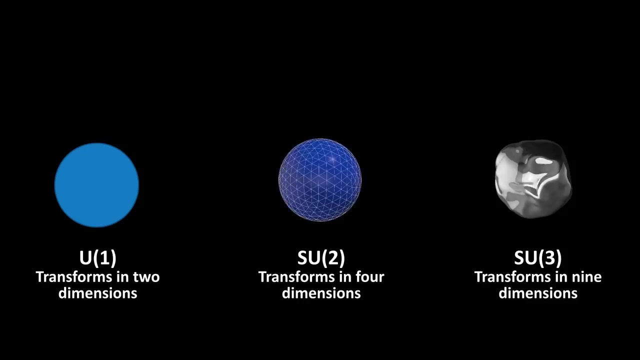 we observe. Now. why do I say mass can only be explained by symmetry? breaking The problem of mass is fundamental to the standard model's construction. At its core, it has three symmetries called U1, SU2, and SU3.. Each symmetry is associated with a fundamental force of nature. 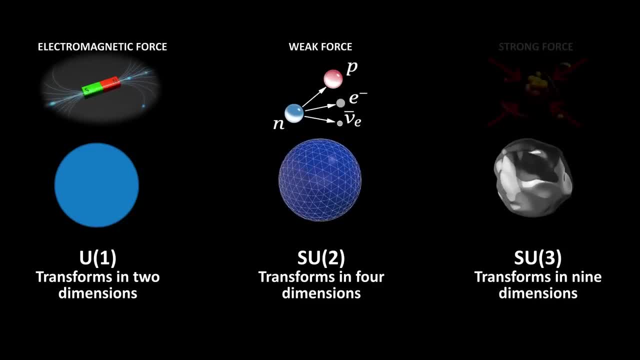 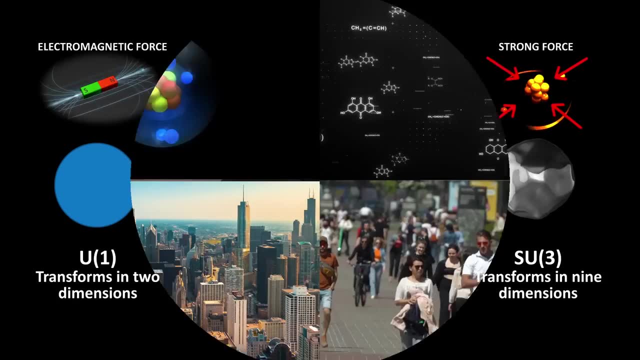 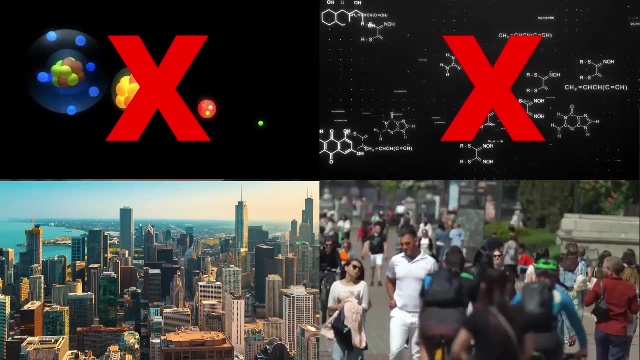 namely the electromagnetic weak force and strong force resistance. In other words, these symmetries result in three of the four fundamental forces. These form the basis of the universe we live in. Without them, there would be no nuclei, no atoms, no chemistry, no structures of any kind and certainly no life as we know it. 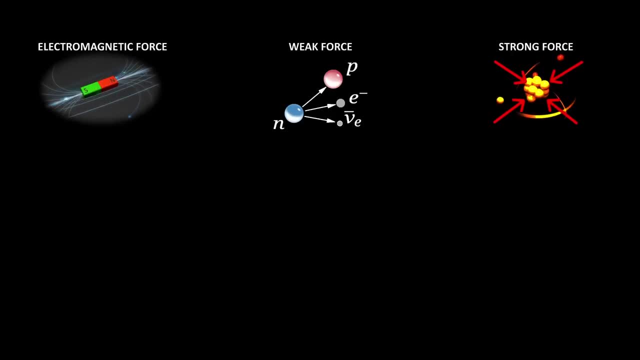 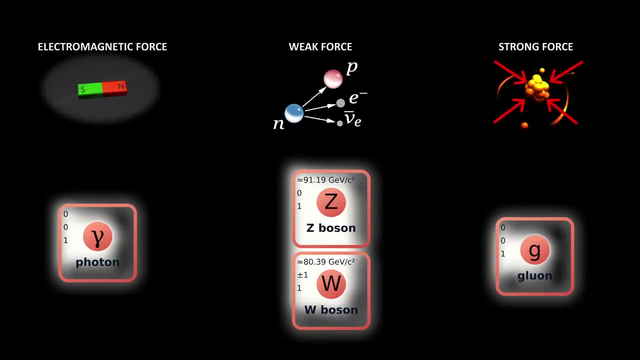 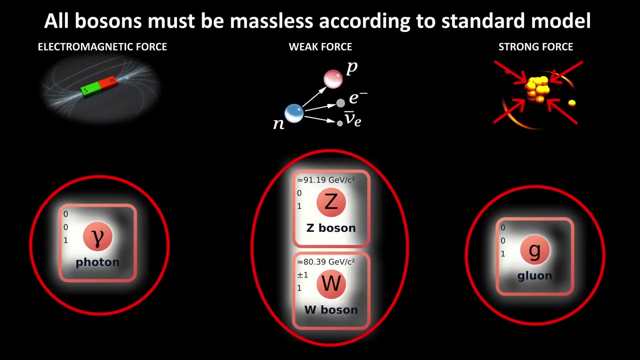 And these forces in turn are mediated by force carrying particles, namely the photons in electromagnetism, the W and Z bosons in the weak force and gluons in the strong force. Now here is the issue. These particles must all be massless according to the equations of the. 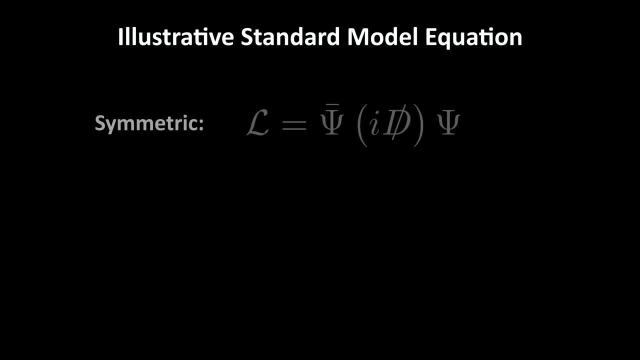 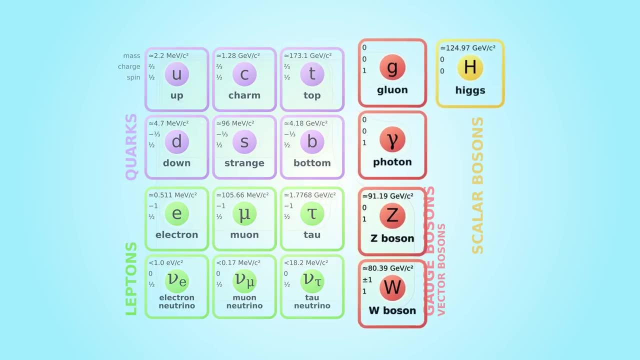 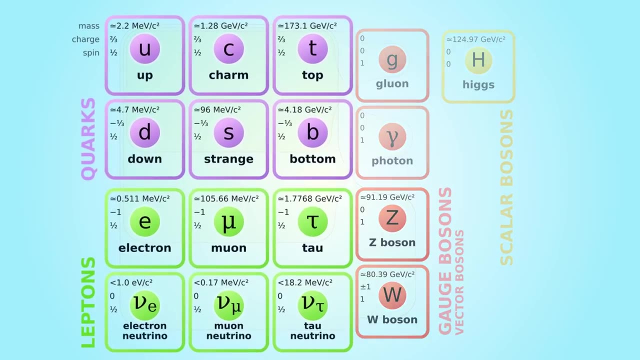 standard model. This is a demand from the symmetry of the equations. They give you massless bosons, not massive bosons. This also includes the Higgs boson. It must also be massless according to the equations. Furthermore, since all matter particles called fermions, 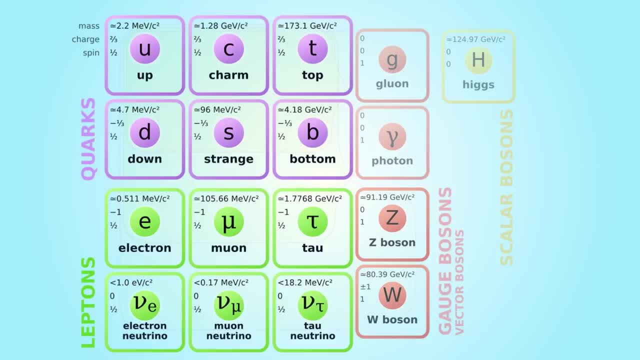 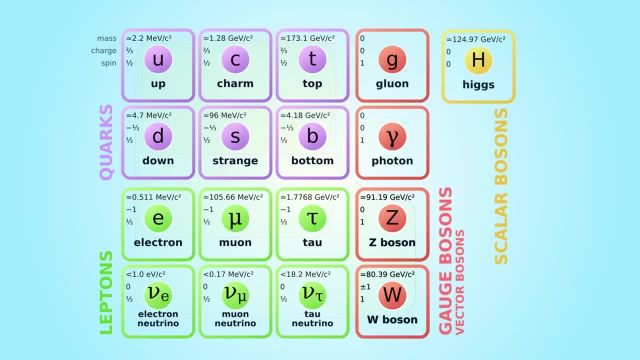 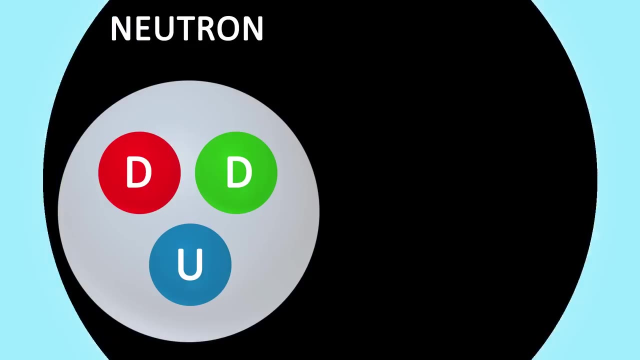 also get their mass from the Higgs field, fermions would also be massless. This is clearly not the case, because fermions do have mass And in the case of bosons, the theory describing the weak force can only work if the W and Z particles have mass. Why This has to do with the fact that the 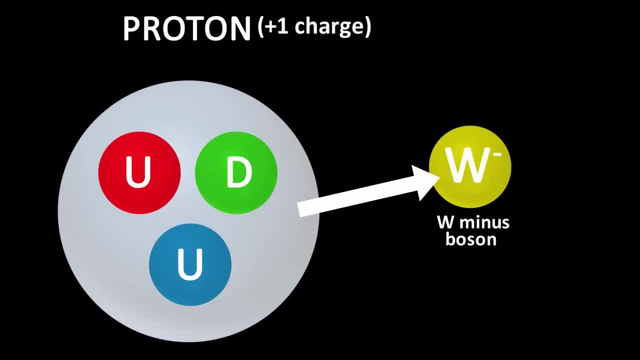 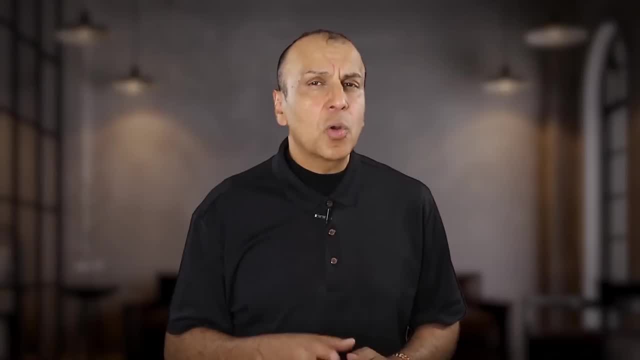 weak force has a very limited range. If W and Z bosons were massless, they would work like electromagnetism with unlimited range. But that's not how they work. So how do masses of the fundamental particles come about? They come about due to the Higgs mechanism. 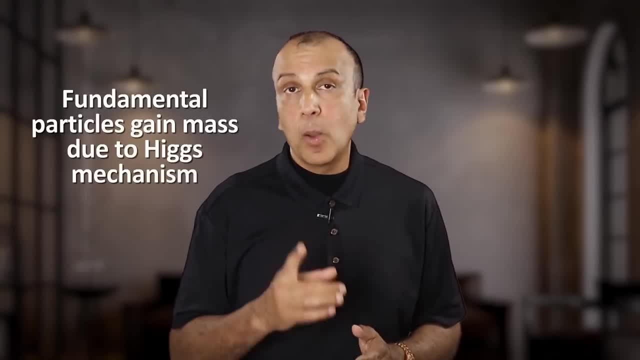 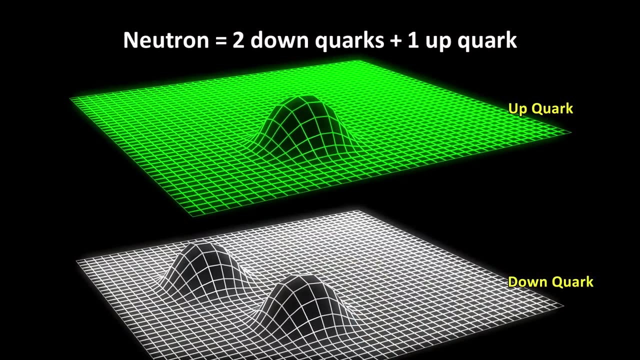 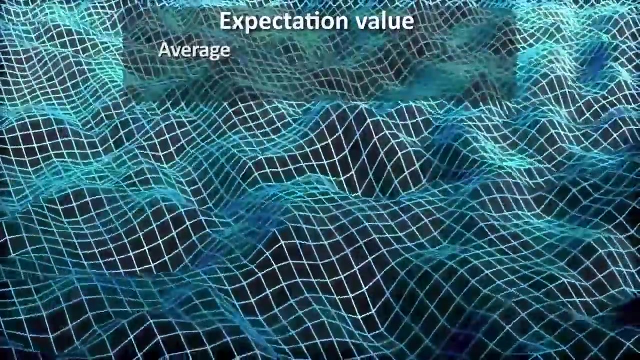 Which is a result from symmetry breaking. What do I mean? Briefly, modern quantum theory shows that all particles are excitations and fields that permeate the entire universe. The vacuum expectation value of these fields is zero. Expectation value is the average of all possible measurement outcomes weighted by their 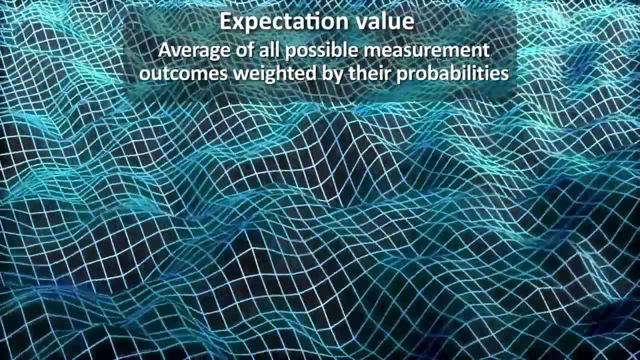 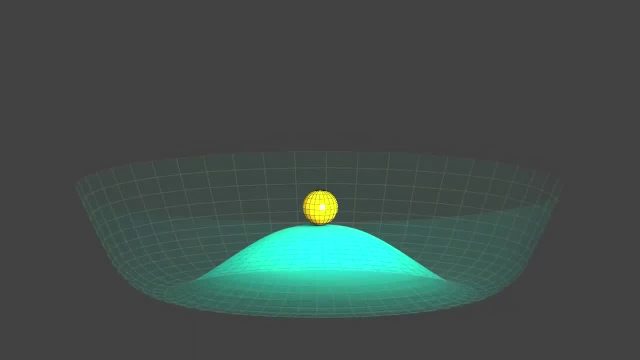 probabilities Zero would be the expected value of all these quantum fields. This is a difficult concept to understand, but it is a very important concept to understand. It is a very important concept to understand, so let me explain this another way. The Higgs field is a little. 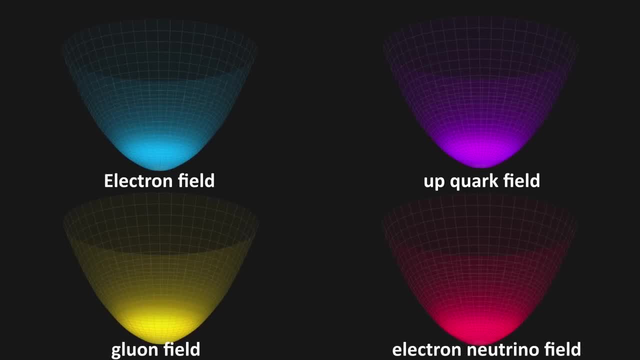 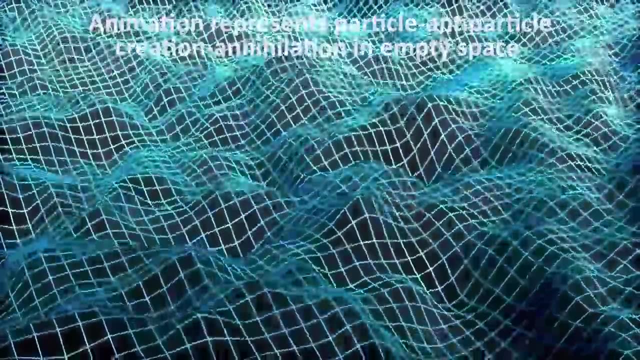 different than every other field. The difference is that the lowest energy state of all the other fields is zero. This means that, even though they are modulating and changing meaning, the particle and antiparticles are quickly coming in and out of existence, forming and. 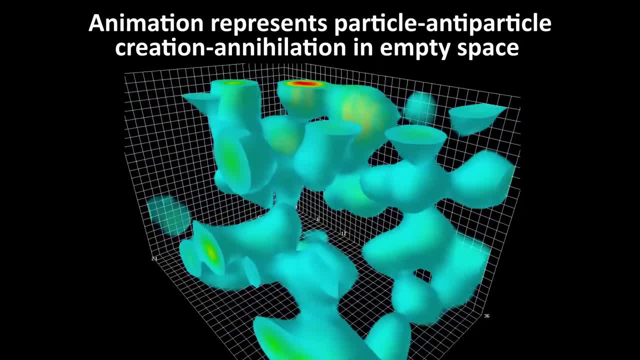 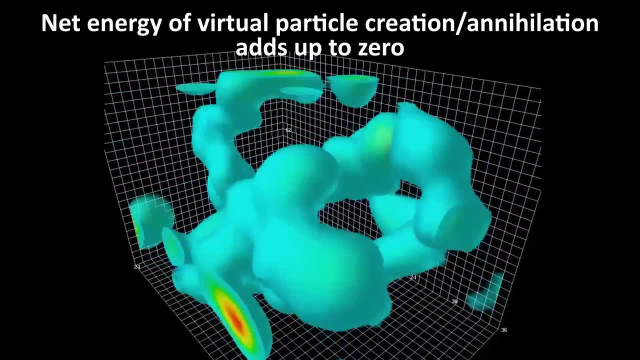 annihilating all the time. all the energy used to create these virtual particles, which are then annihilated, adds up to a net energy value of zero. The universe registers this as a zero energy state for these fields, But the Higgs field is different. It is: 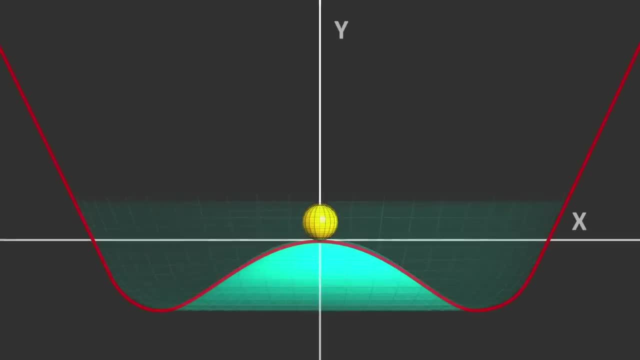 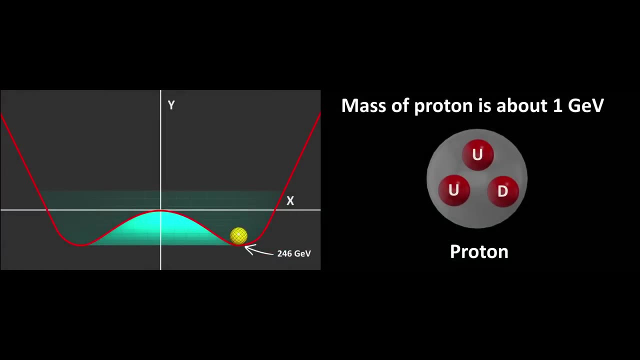 non-zero even in empty space. It is in fact 246 gigaelectron volts, or GeV. To give you a meaningful comparison, the energy or mass of a proton is only about 1 GeV. Going back to our 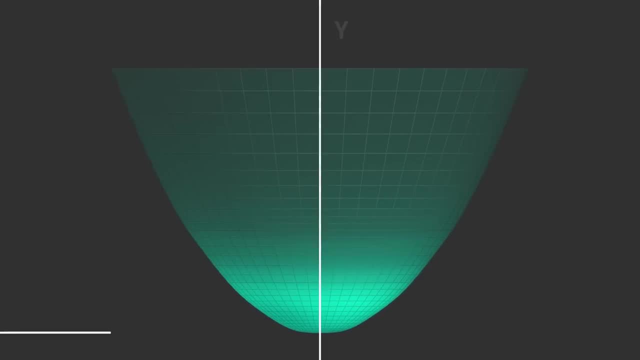 Mexican hat potential. the x-axis represents the expectation value, the y-axis is potential energy and the ball represents the Higgs field. When the theory is written in a symmetric state, like where the ball is in the center, again the ball represents the Higgs field, the expectation. 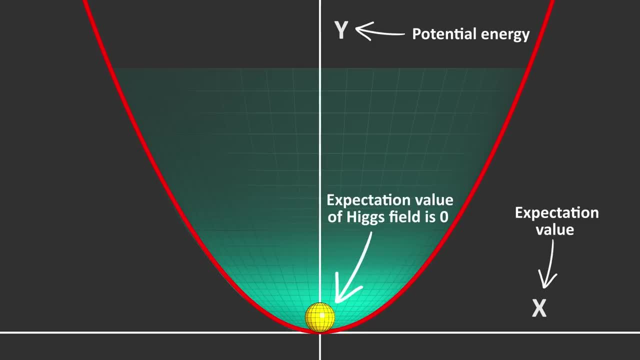 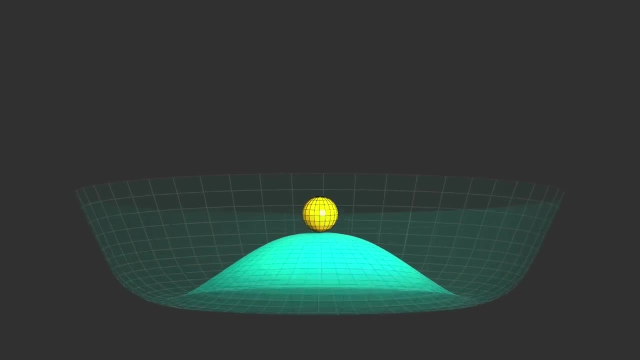 value of the Higgs field in this state is 0. Everything is massless at this point. This was the case in the early universe, when the energy and temperatures were much higher. But at a lower temperature the energy potential of the Higgs field changed. That is the ball dropped. 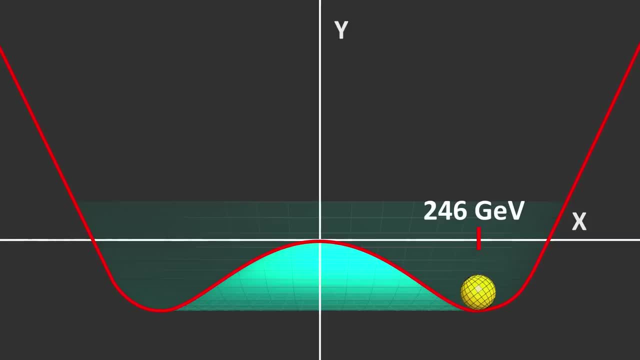 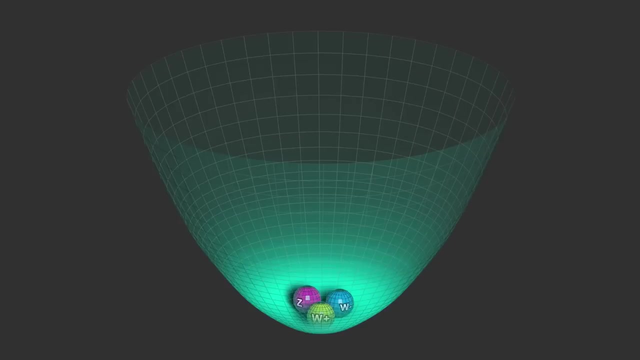 energy point. This is where we are today. The Higgs field has an even lower energy point where the expectation value is non-zero. This breaks symmetry. This means our Higgs field becomes massive at this lower energy state. What this means is that any fundamental particle that interacts with the Higgs field at this 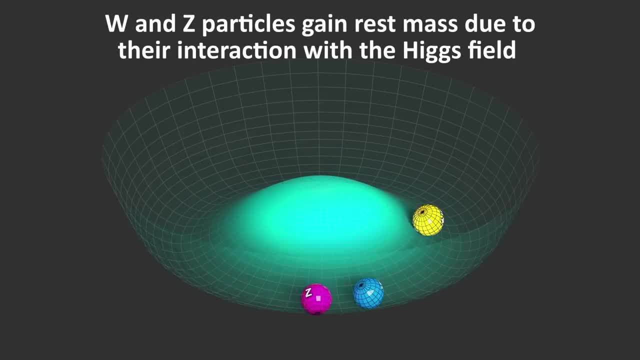 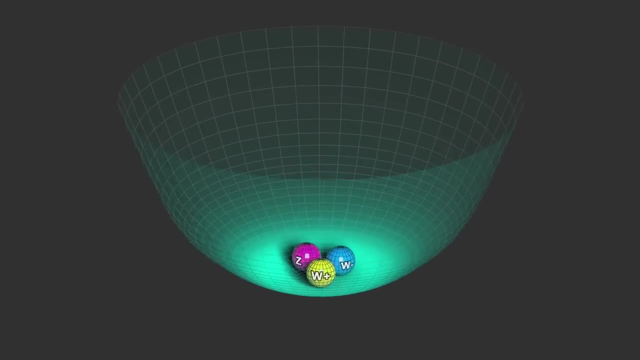 non-zero potential gains a rest mass. All the mass associated with the particles of the standard model is due to the fact that they interact with the Higgs field. Particles that don't interact with the Higgs field remain massless, like the massless photon. This is the so-called Higgs mechanism and is the way in which 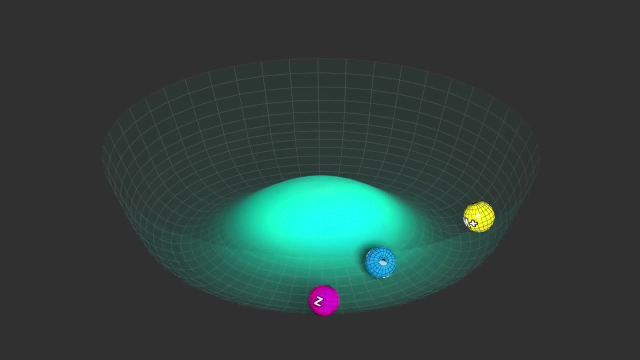 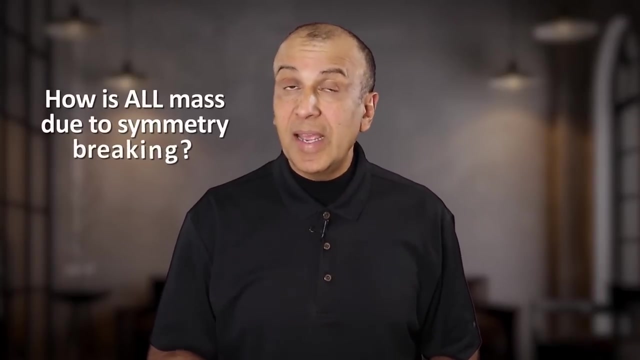 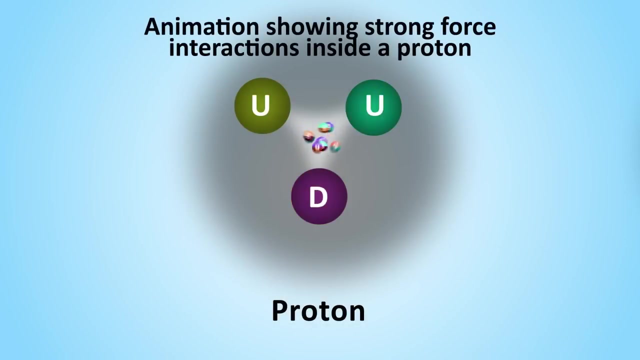 certain symmetries of the standard model are broken spontaneously to impart mass to fundamental particles. But I stated that all mass is due to symmetry breaking, not just the mass of fundamental particles. How is that explained? The Higgs field does not explain most of the mass in the universe, The mass of protons and neutrons, which are 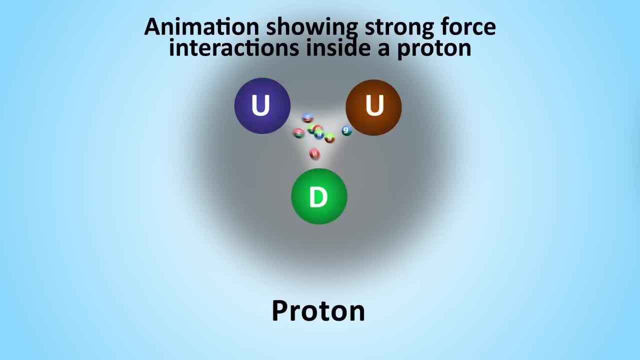 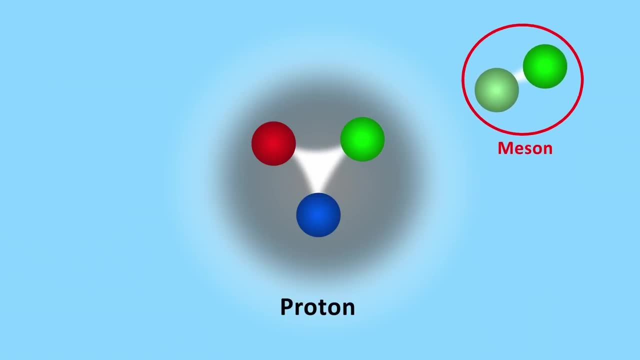 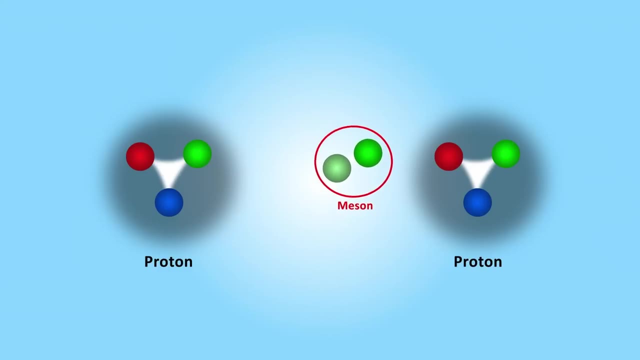 almost the entire mass of atoms comes mainly from the binding energy that keeps quarks glued together inside protons and neutrons, as well as the binding energy that keeps protons glued to other protons and neutrons in the nucleus. Put another way, it comes from gluon interactions associated with the strong. 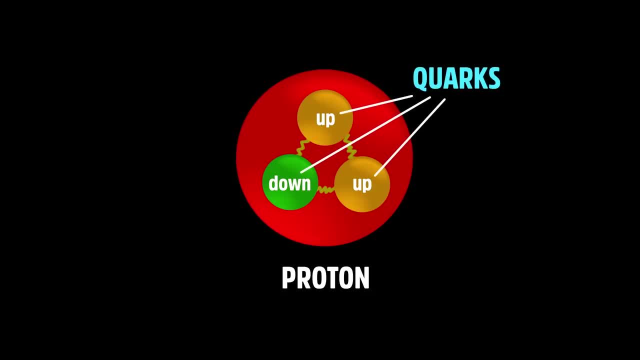 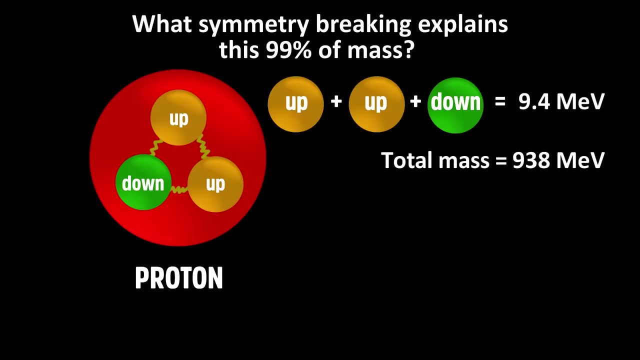 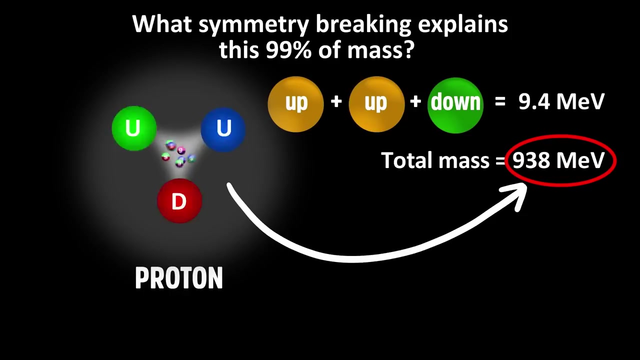 force. If you add up the mass of all the fundamental particles that make up atoms, it would only amount to about one percent of their mass. 99% of the mass comes from binding energy, due to the strong force. Now the question is what kind of symmetry breaking explains this binding energy? 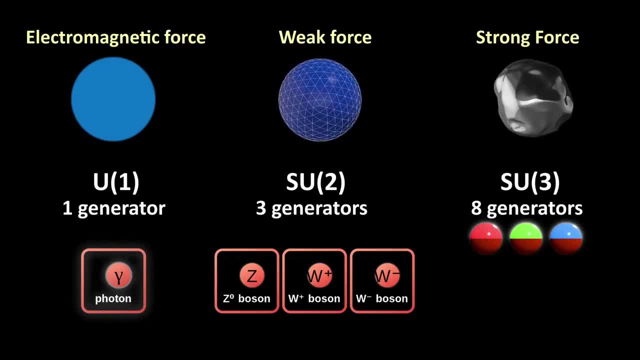 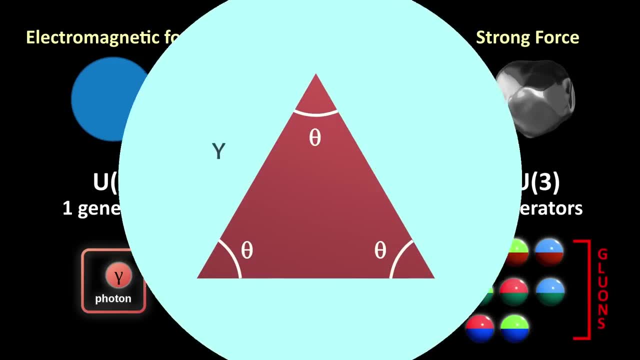 It turns out that, other than the gauge symmetries or force symmetries, which give us the three fundamental forces, there are also other symmetries in the standard model. For example, there is chiral symmetry. We can think of this as the symmetry of a mirror image, A chiral. 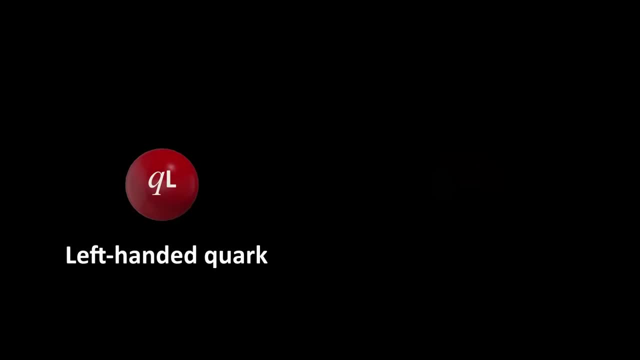 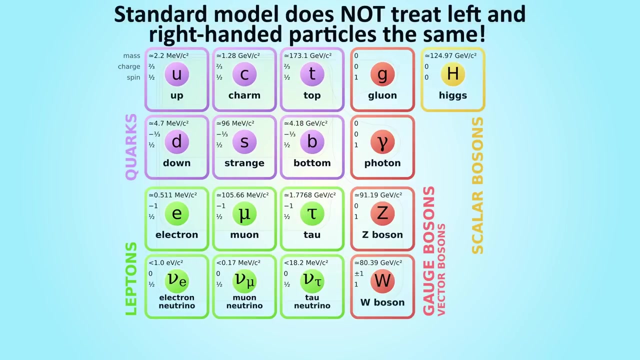 symmetric theory treats left-handed and right-handed particles the same. For example, in such a theory, if we swapped a left-handed particle in any reaction with a right-handed particle, nothing would change. But the standard model is a chiral theory, meaning that it does NOT. 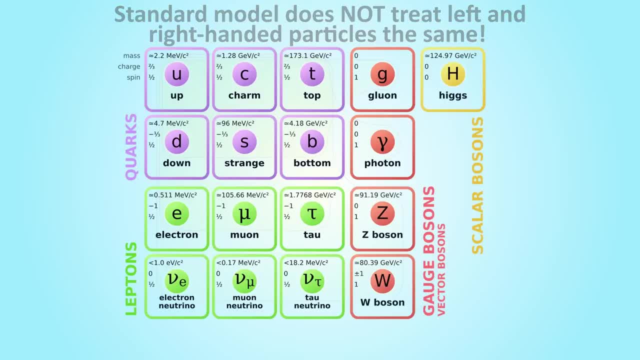 treat left and right-handed particles the same. For example, the weak force only acts on left-handed, not right-handed particles. In addition, as far as we know, only left-handed handed neutrinos exist. Right handed neutrinos have never been detected. 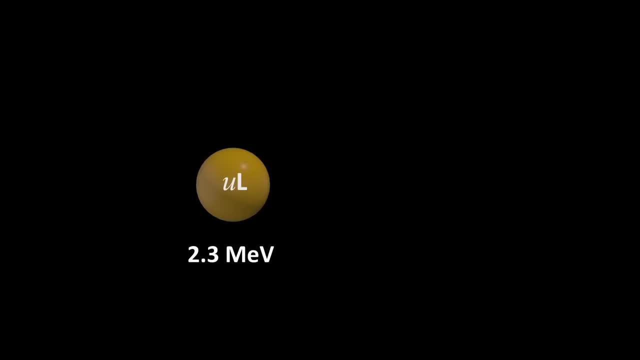 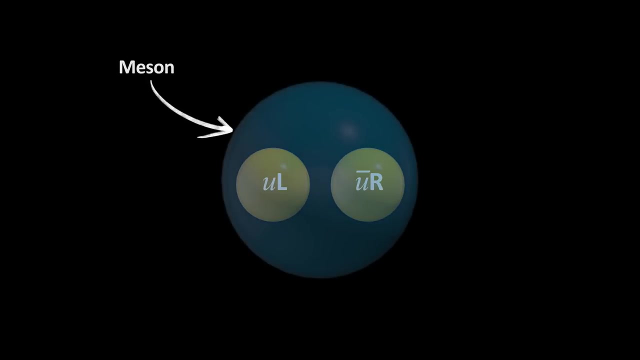 Consider a left handed up quark. It has a mass of around 2.3 MeV. Now consider the antiparticle of this quark. Since it's an antiparticle, it will be right handed When these two quarks are bound together. this combination is called a meson If left and right 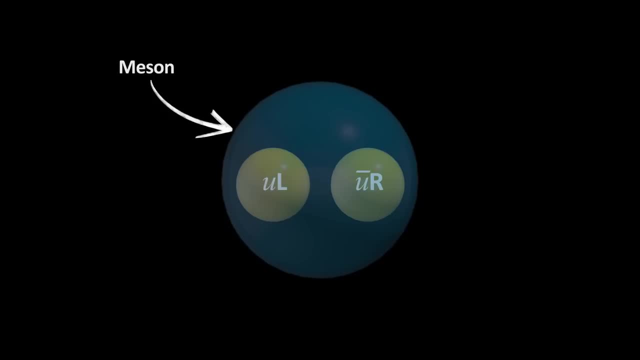 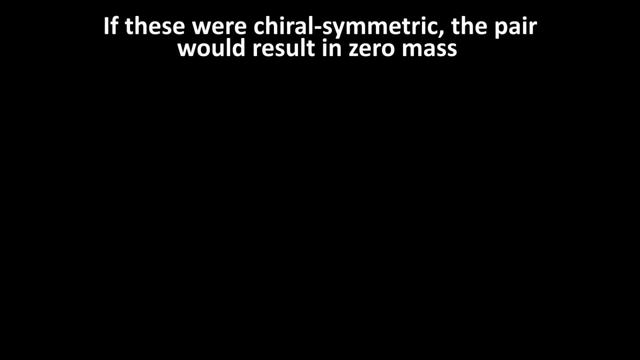 chirality were treated equally, this meson would annihilate, with a net energy of roughly zero. In other words, the combination of a quark-antiquark pair would result in zero mass. However, if chiral symmetry is broken, they are not treated equally and the net energy is not. 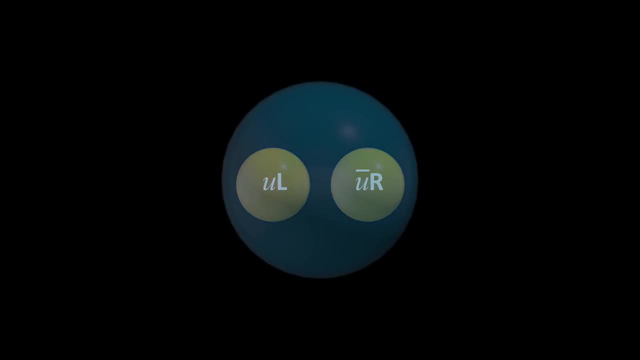 zero. In fact, something remarkable happens to the mass when these two particles are bound together by gluons. The total mass is not zero and it's not 4.6 MeV. If you were adding the individual meson, it would be 0.5 MeV. If you were adding the individual meson, it would be 0.5 MeV If you. 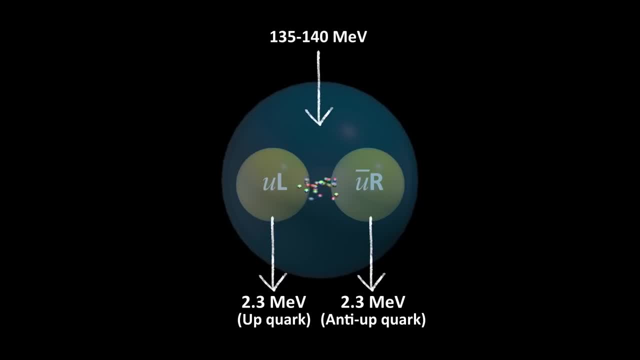 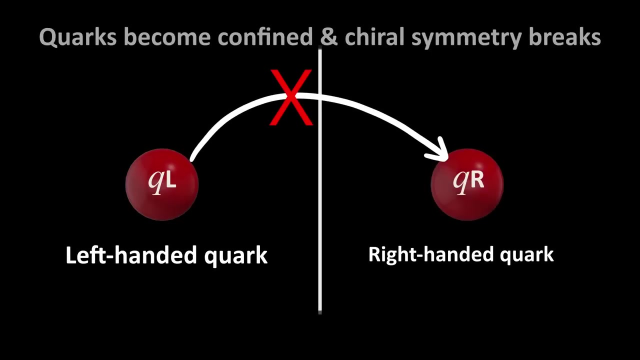 were adding the individual meson, it would be 0.5 MeV, But a whopping 135 to 140 MeV. Where did this increase in mass come from? It comes about due to chiral symmetry breaking As the quarks become confined by the strong force via the exchange of gluons. 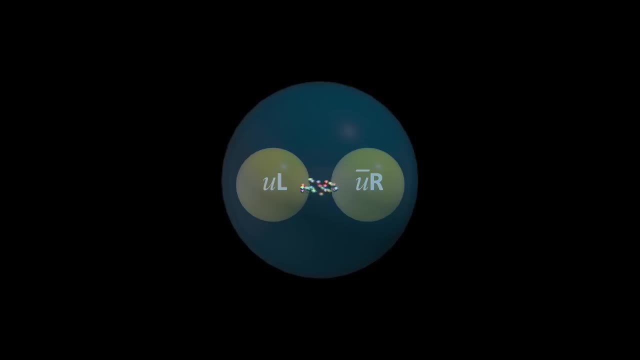 chiral symmetry breaks The gluons form a kind of cloud around the quarks. This confines the quarks, breaks chiral symmetry and generates the binding energy that is measured as mass of the meson. This same phenomenon occurs in protons and neutrons. 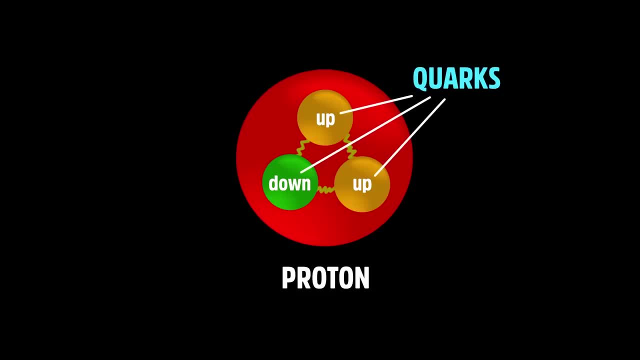 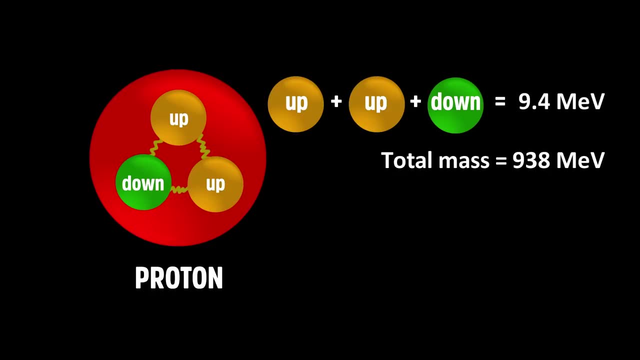 So, for example, in a proton, if you add the individual masses of the three constituent quarks, it adds up to only 9.4 MeV. But the actual measured mass of a proton is 938 MeV, a difference of nearly 100x. The additional mass is due to chiral symmetry breaking. 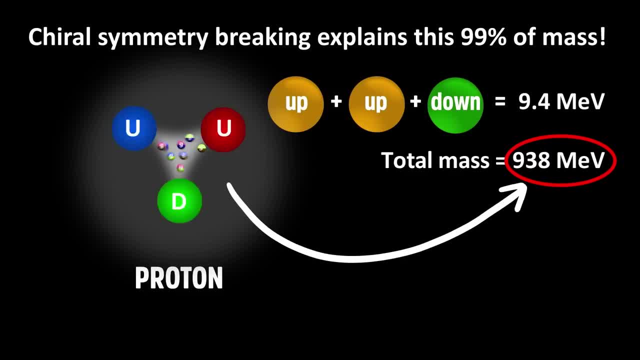 from the gluon-cloud interactions. This is the origin of 99% of the visible mass of the universe. The other 1% is due to the mass of fundamental particles from the Higgs boson. We can visualize the symmetry breaking of quarks. 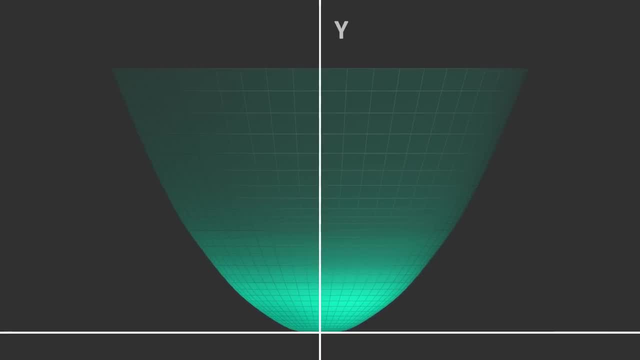 in a similar way as the symmetry breaking of the Higgs field. At a high energy state, such as the one that existed in the early universe, the expectation value for the quark anti-quark pair was zero. This is the state where chiral symmetry existed, But as the universe cooled, 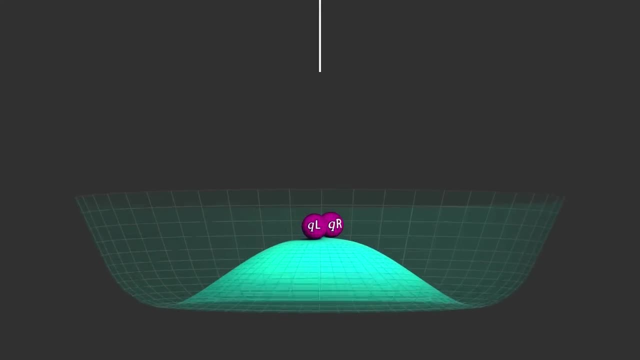 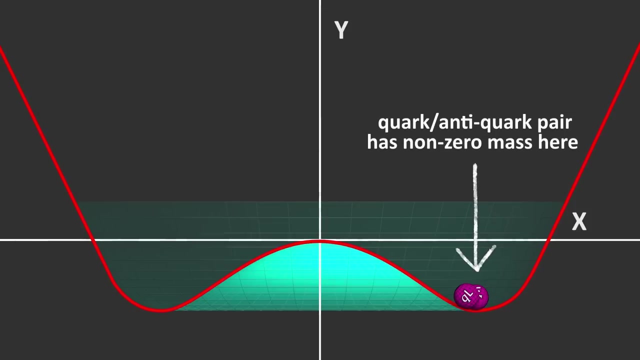 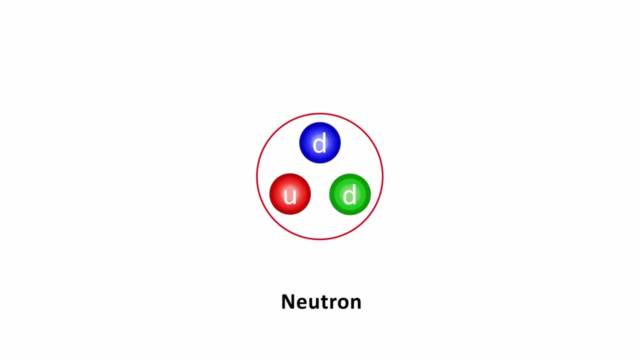 to the energies of today, this symmetry was broken and today the result is that quark anti-quark pairs have a non-zero mass due to the gluon-cloud around quarks. Now I want to point out that this is the cutting edge, best explanation we have today of how. 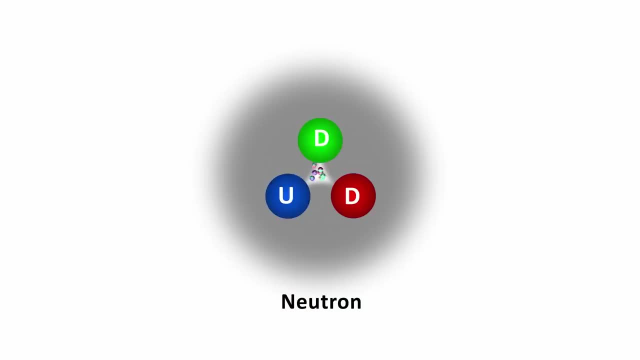 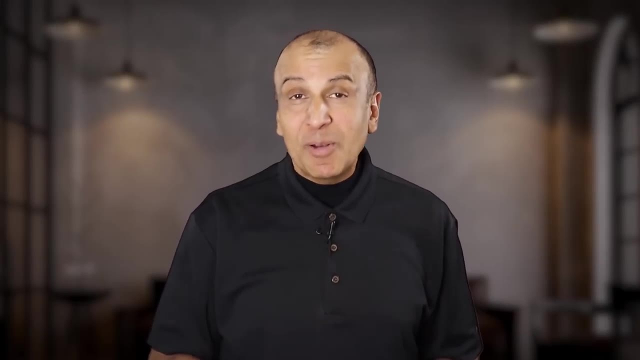 mass comes about. But you should know that this is an active area of research where the details are still being worked out, So we are going to learn a lot more in the coming years, But if you want to learn a lot more about the subtle science that we do know, I highly recommend a 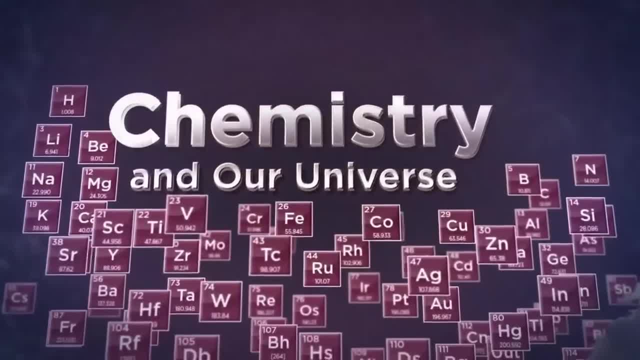 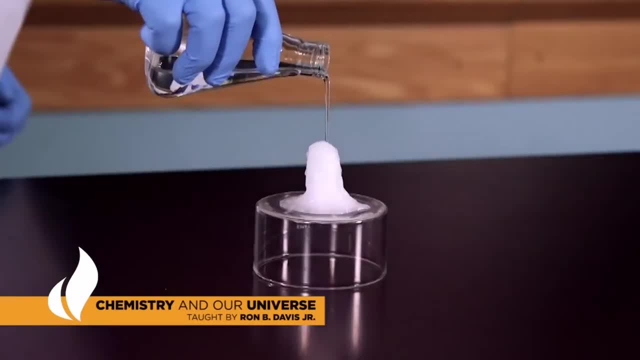 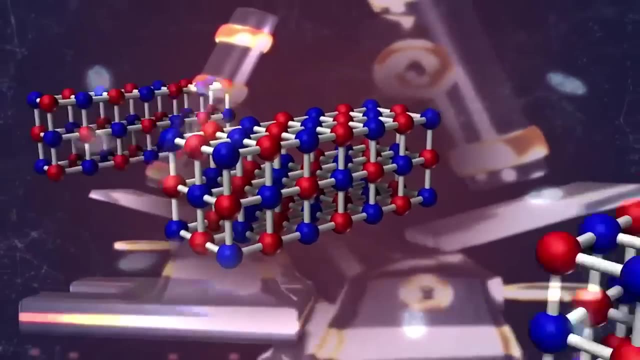 lecture series available on Wondrium. today's sponsor called Chemistry and Our Universe- How It All Works. It's a 60-part college-level course from award-winning chemistry professor Ron Davis of Georgetown University. If you want to know why matter behaves the way it does, then 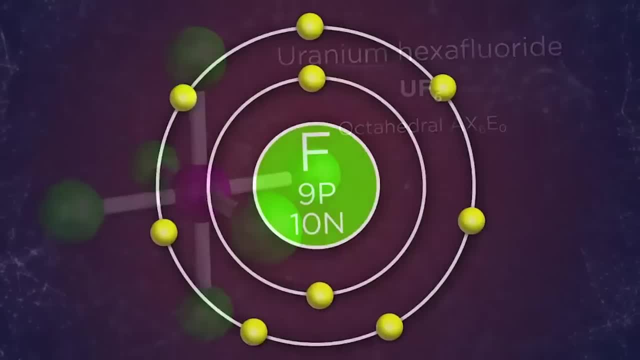 you'll want to check this out. Professor Davis first walks you through the foundational principles of chemistry via graphically. He will explain why matter behaves the way it does and how it works. Professor Davis first walks you through the foundational principles of chemistry via graphically. 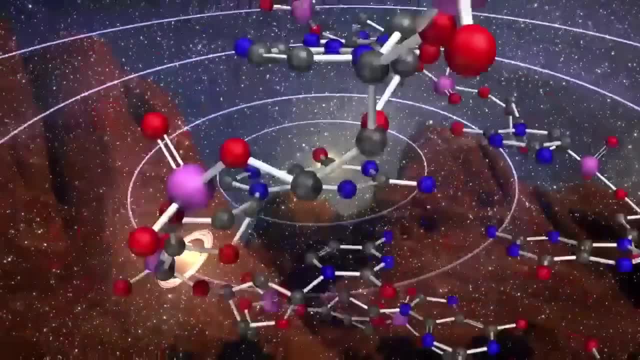 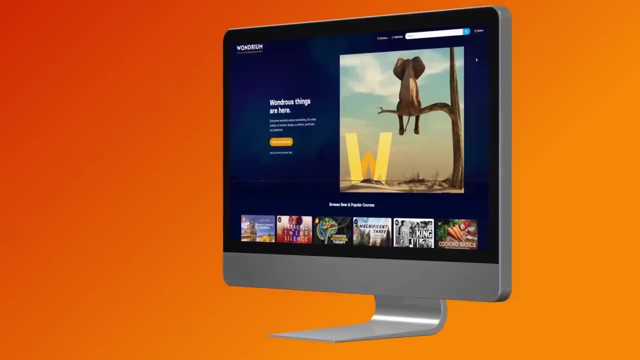 Professor Davis first walks you through the foundational principles of chemistry via graphically, Then he shows you how those concepts can be used to explore the universe, from the Earth to the stars, to the human body. You'll find this and many other wonderful courses on Wondrium taught by some of the best educators in the world. That's why I've been a member of